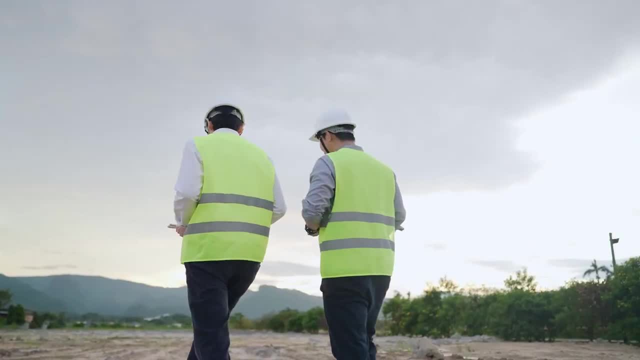 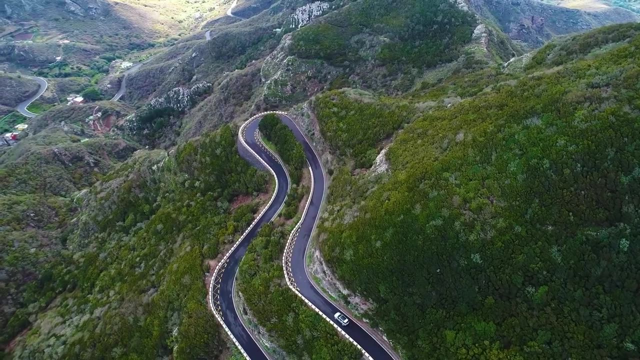 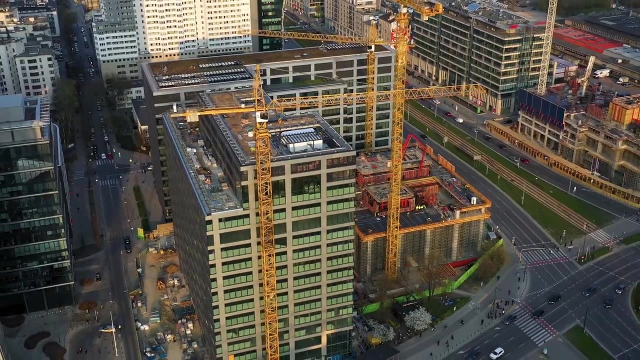 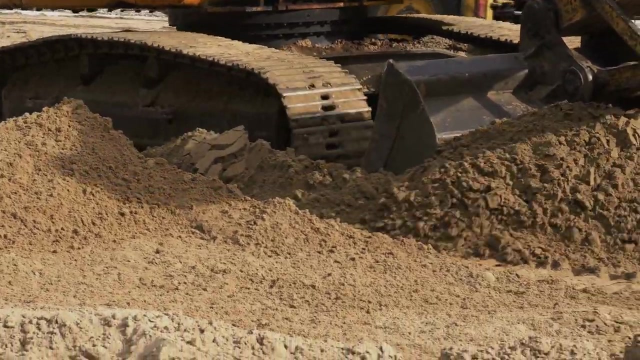 common composition and characteristics. The investigation provides valuable insights to engineers, helping them design safe and efficient foundations, slopes, retaining walls and other structures. Consider the construction of a high-rise building in an urban area. The soil conditions at the site may include soft clay layers mixed with sand and rock at various 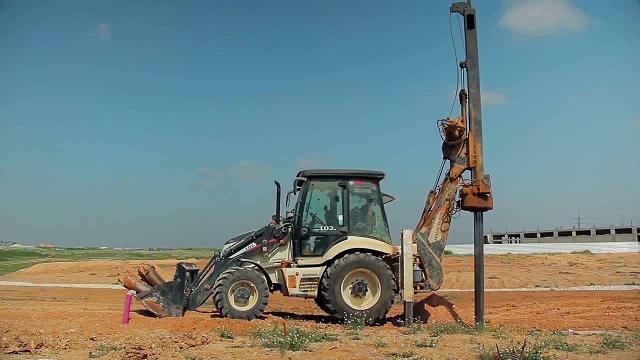 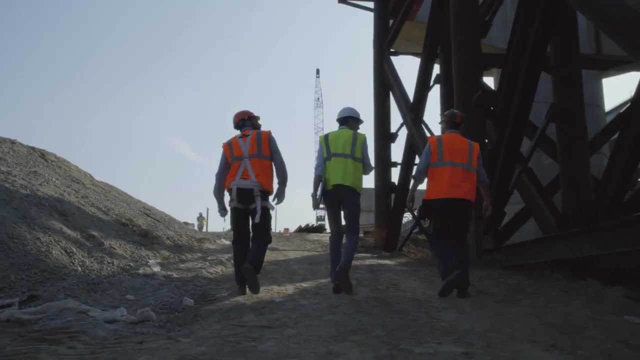 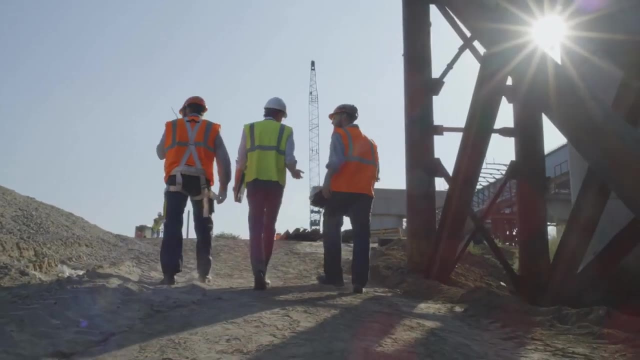 depths. Without a proper geotechnical investigation, the foundation may be a little bit more difficult. The structure may not be designed to handle the building's weight or resist the forces generated during an earthquake. By conducting a thorough investigation, engineers can determine the most suitable foundation type for the structure to transfer its load to a more stable. 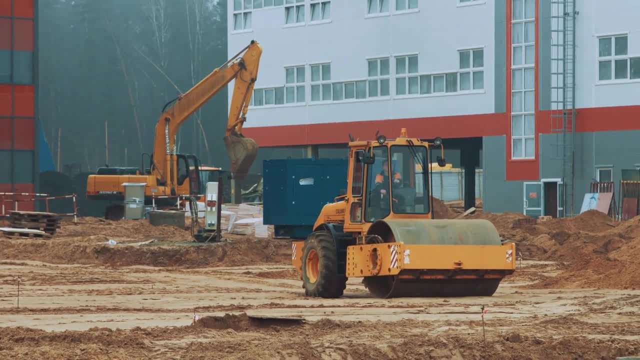 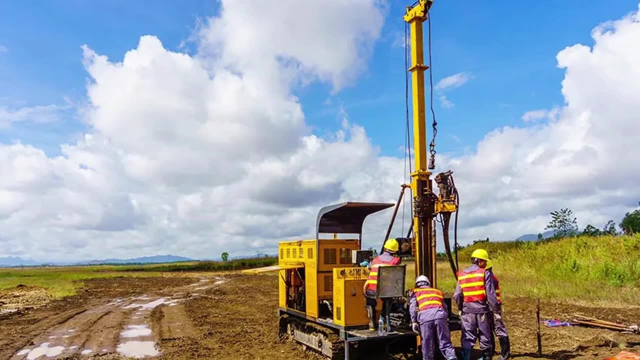 layer Also suggest ground improvement techniques such as soil compaction or grouting to enhance the soil's strength and reduce settlement. A thorough geotechnical investigation is vital and for several reasons, which includes safety, knowing the soil's properties and knowing the 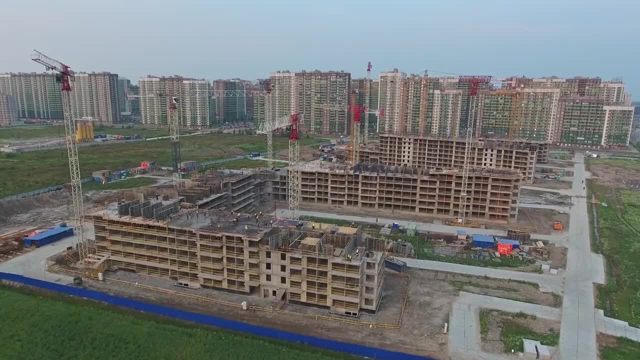 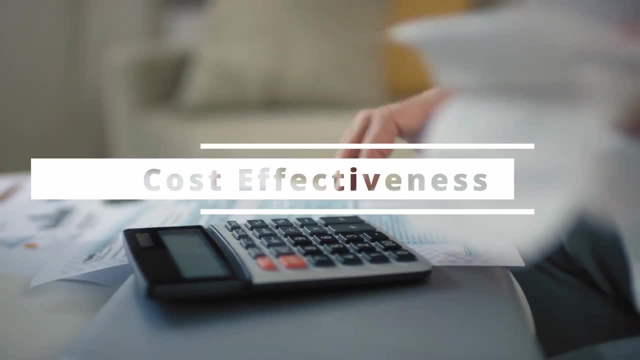 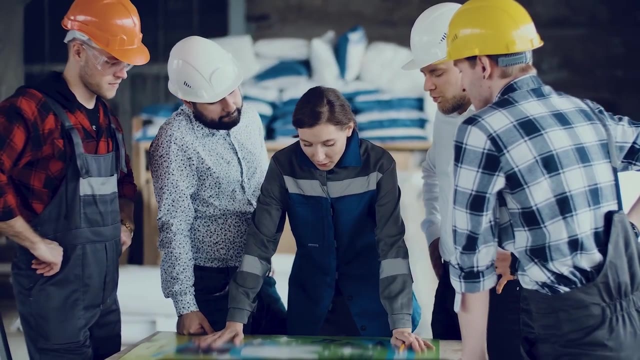 soil's properties helps engineers design foundations that can support the weight of the structure and resist natural hazards such as earthquakes, landslides and soil liquefaction. Cost-effectiveness: By understanding the soil conditions, engineers can select the most suitable construction techniques and materials. 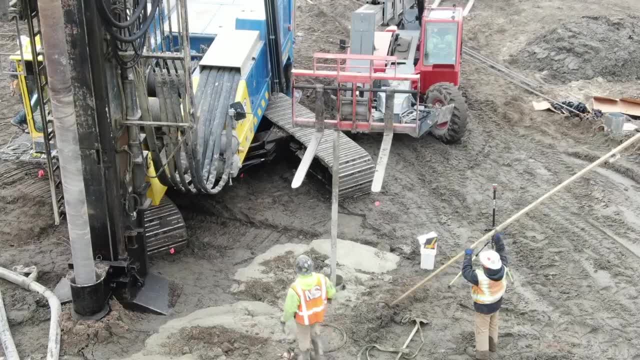 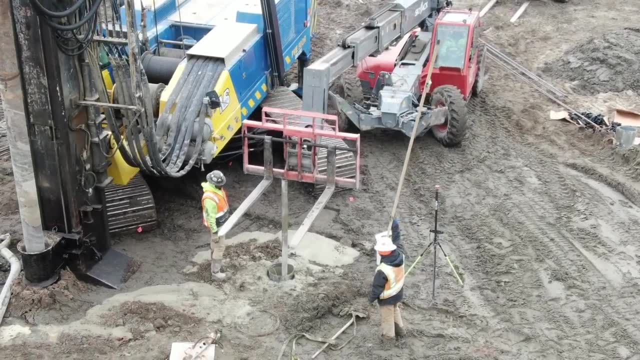 which can save time and money in the long run. Environmental protection- Geotechnical investigation- helps identify and mitigate potential environmental impacts, such as groundwater contamination and water pollution. Environmental protection is a key element in the construction of a project, and it is also a key element in the construction of a project. 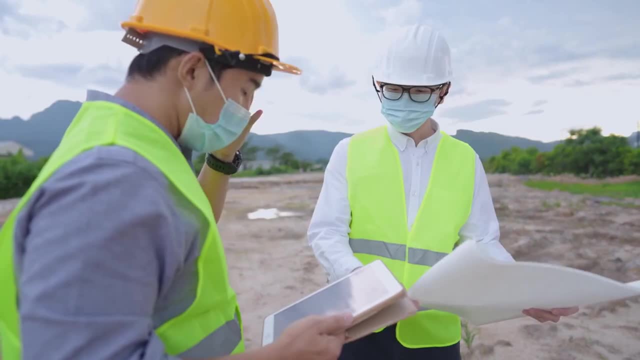 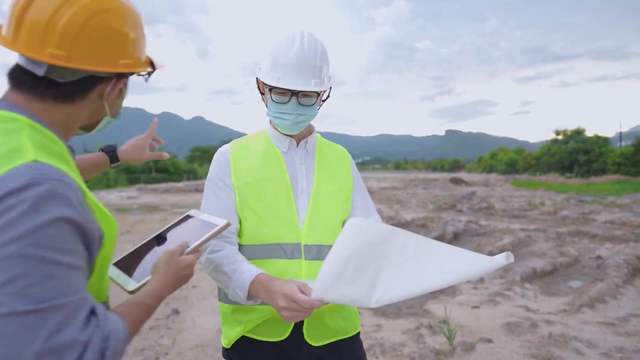 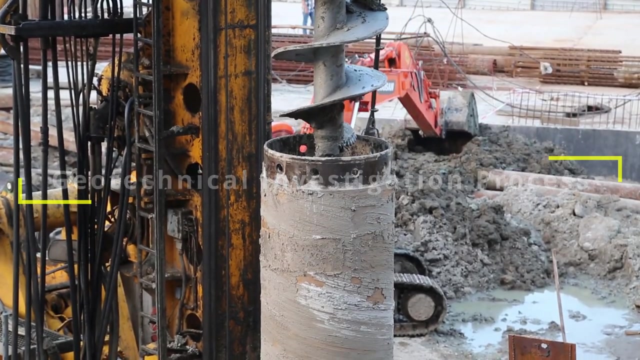 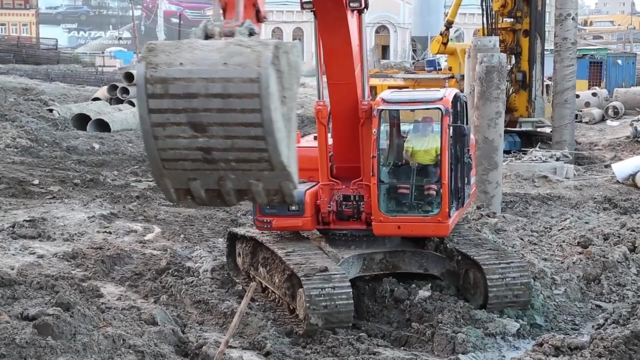 Legal compliance. In many jurisdictions, conducting a geotechnical investigation is a regulatory requirement to ensure that construction projects meet safety standards and environmental regulations. Geotechnical investigation involves several steps, which can vary based on the project's size and complexity. Here's a general overview of what 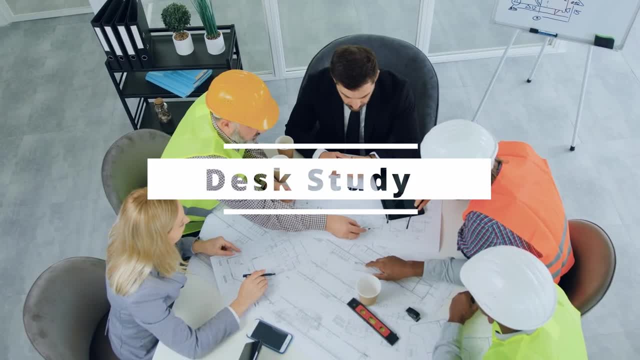 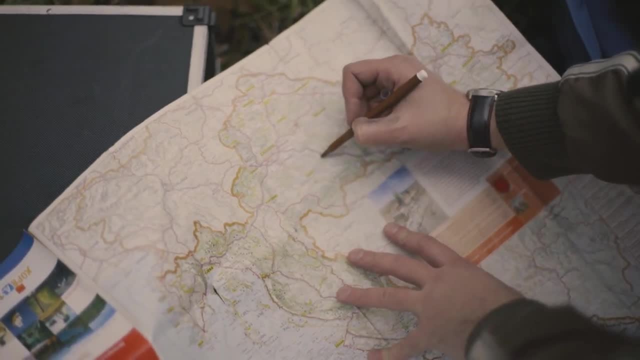 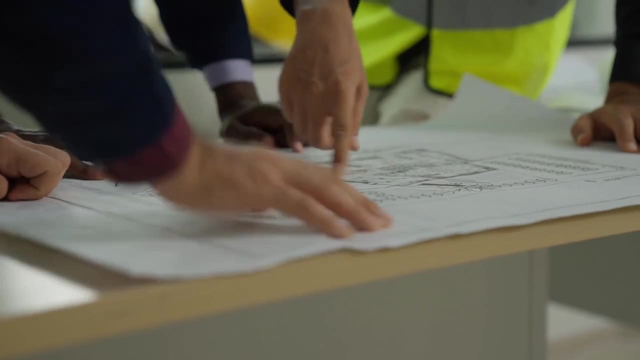 those steps look like Desk study. This preliminary research involves collecting existing data about the site, such as geological maps, aerial photographs and historical records. This information helps engineers develop an initial understanding of the site's conditions and identify potential hazards. Site reconnaissance: 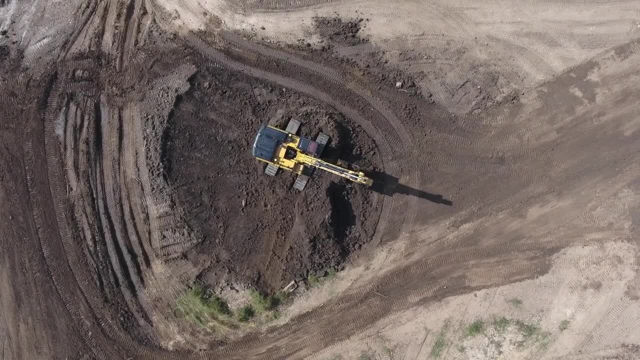 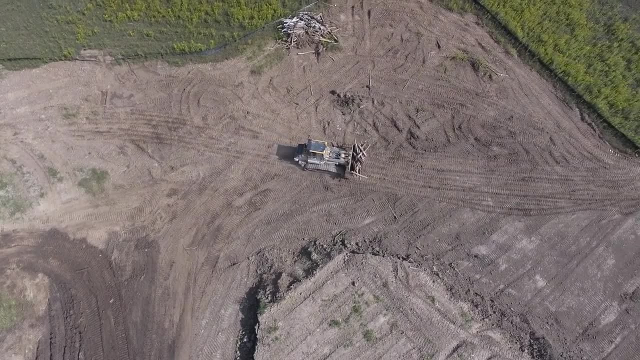 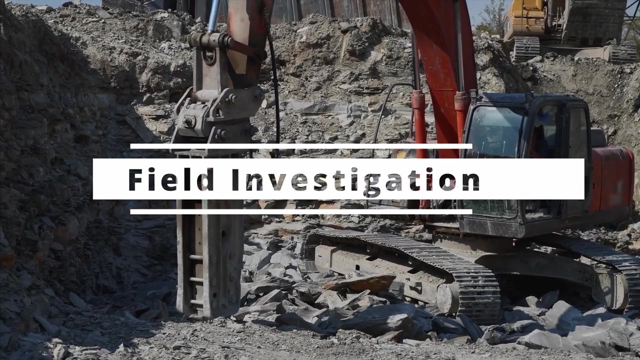 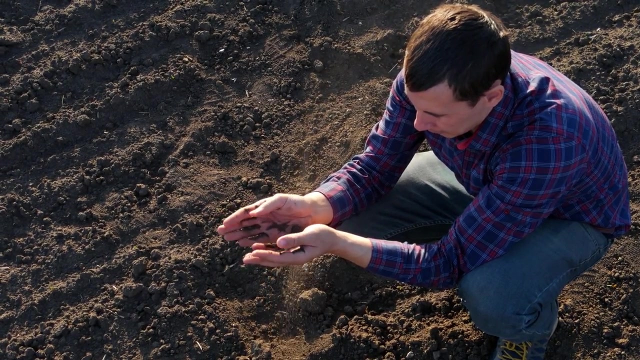 In this phase, engineers visit the site to visually inspect the terrain, vegetation, surface water and any signs of instability or distress. They also look for evidence of past erosion, such as old foundations or utility lines. Field investigation: This is where the real fun begins. Engineers use various Anytime 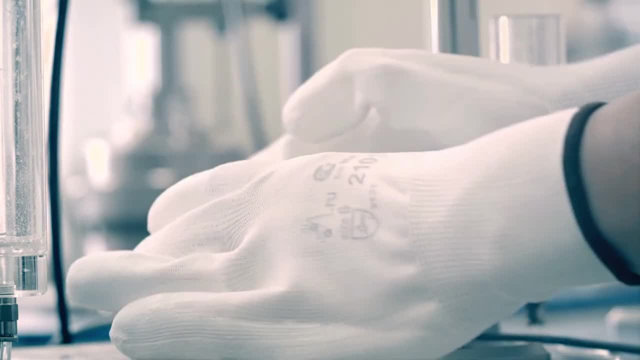 anchore allergies. drunk individuals using optical�라하비―사상��살하와 sea oruty. as subtitles need to be automatically быстрiona ag validate whether they mentioned a爷 Cóired myszysz ul-TTU7a. 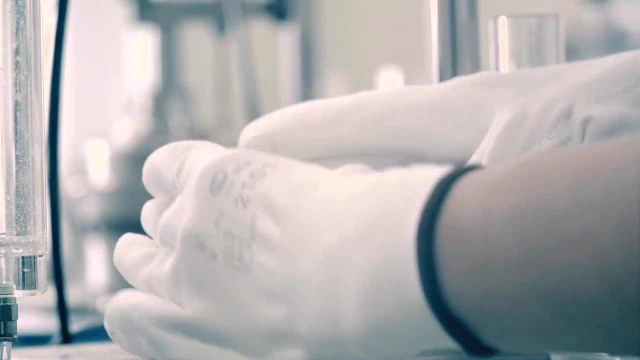 Laboratory testingBill de Carnaval was introduced in each of the two phases in which the samples are collected and are sent to a laboratory where engineers perform various tests to determine the soil's physical and mechanical properties, such as grain size, moisture content, density and shear strength. Vegetable fertilizationkolydiag. Sitting for. 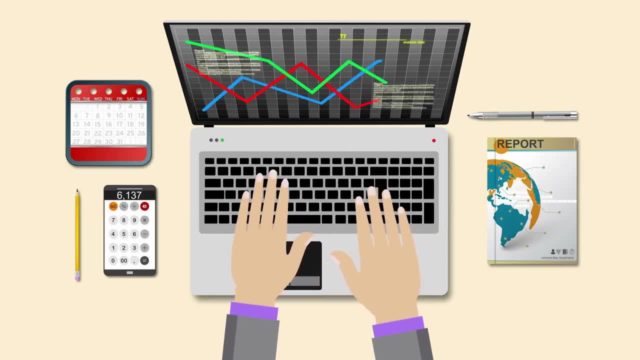 pound, as most soil physician says, survey oil boiler. content этого to Mahereh medo warriors and the sin 실 lorstairمن. in magueo, teachers cook crops to feed their own soil re and report Based on the field and laboratory data, engineers analyze the site's geotechnical. 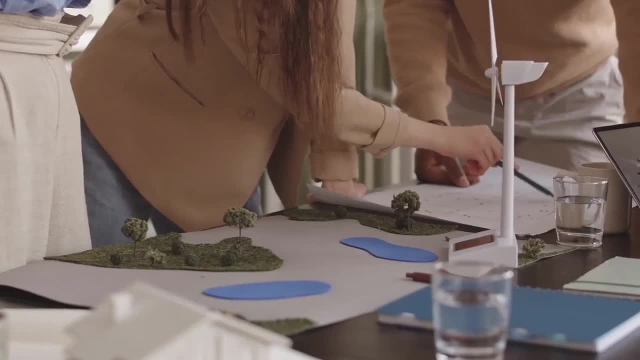 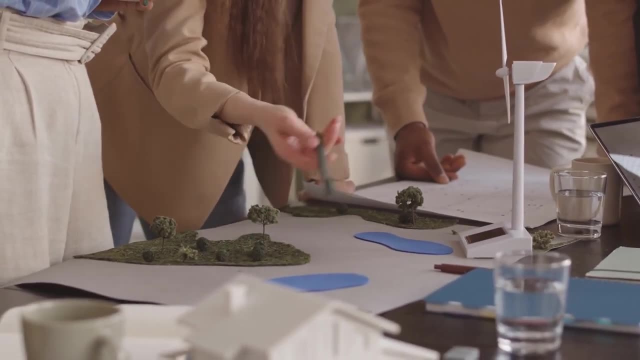 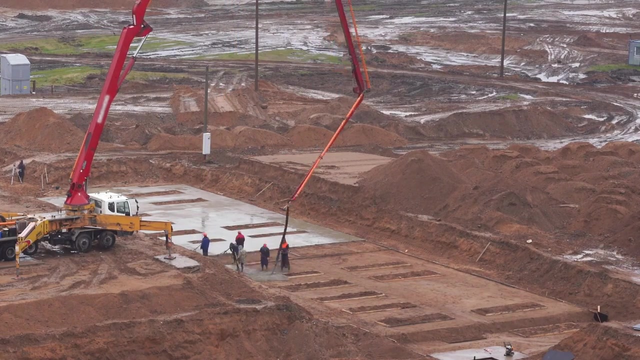 conditions and prepare a comprehensive report. This report includes information on soil stratigraphy, groundwater conditions, soil bearing capacity, settlement estimates and slope stability. It also provides recommendations for foundation design, excavation, support, dewatering and any necessary ground improvement techniques. 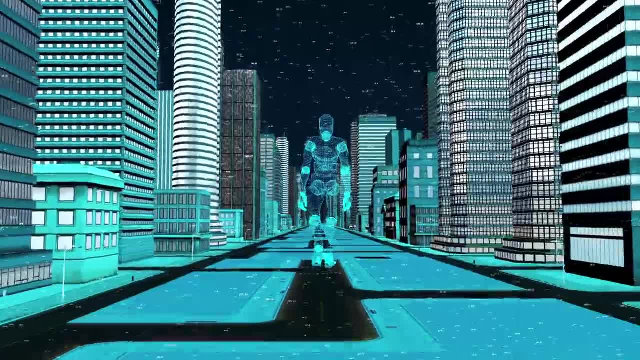 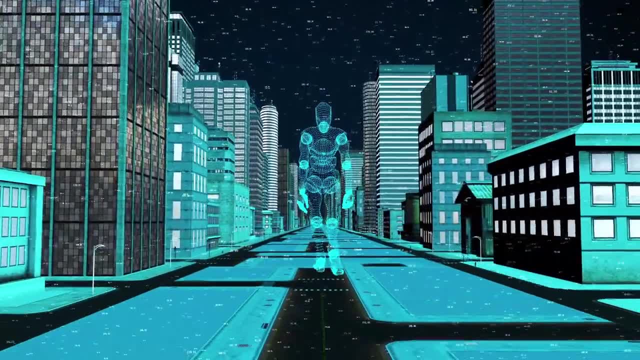 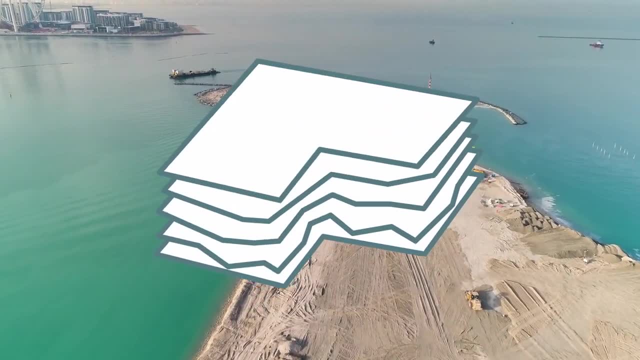 As technology advances, so do the methods and tools used in geotechnical investigation. Some exciting developments in the field include remote sensing techniques like light detection and ranging or LIDAR, and satellite imagery provide high-resolution 3D data about the site's. 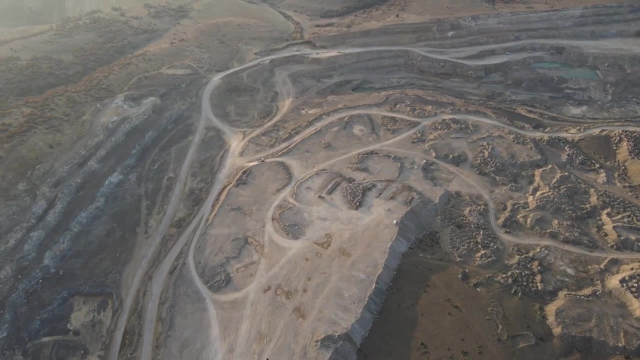 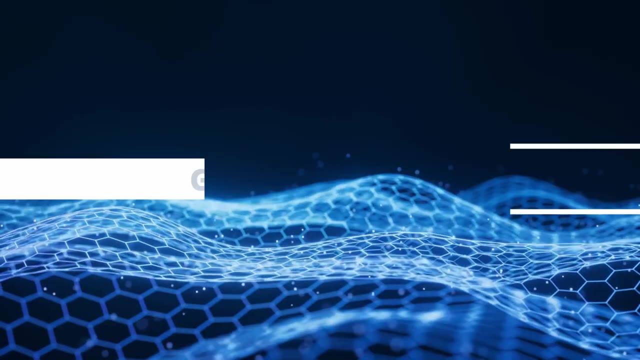 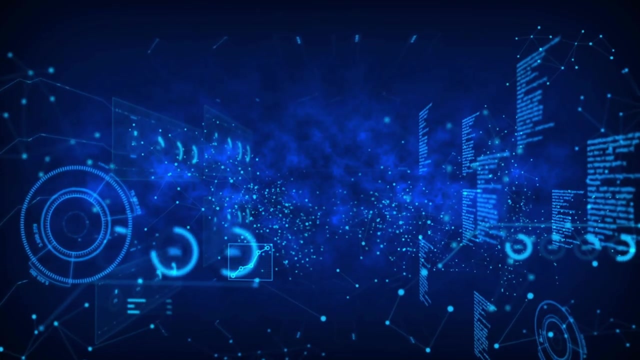 topography. This information is valuable for identifying potential hazards and designing access, roads, drainage systems and other necessary infrastructure. Geophysical methods, Non-invasive techniques like seismic refraction, ground-penetrating radar and electrical resistivity imaging allow engineers to. 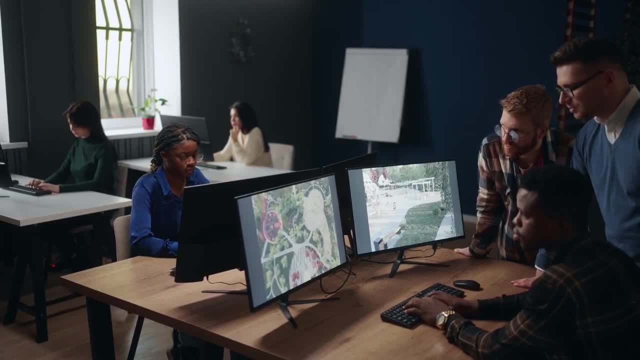 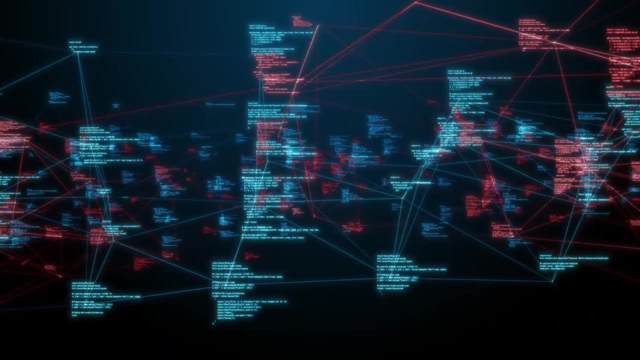 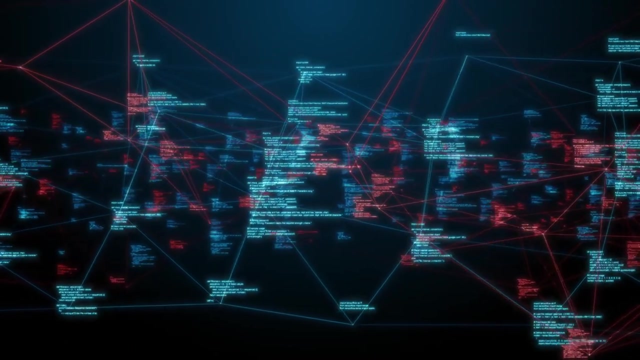 create detailed subsurface profiles without the need for extensive drilling or excavation. Machine learning and artificial intelligence, Advanced algorithms and data processing tools can help engineers analyze vast amounts of data, identify patterns and trends and make more accurate predictions about the site's geotechnical. 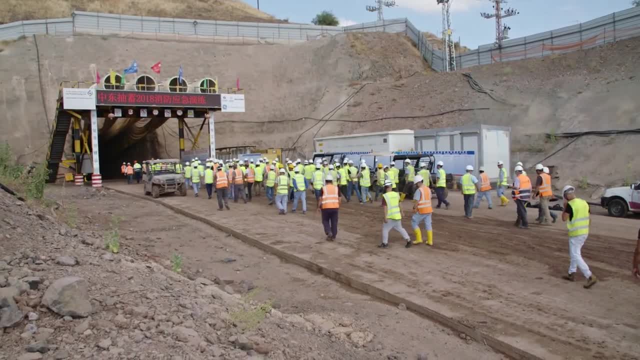 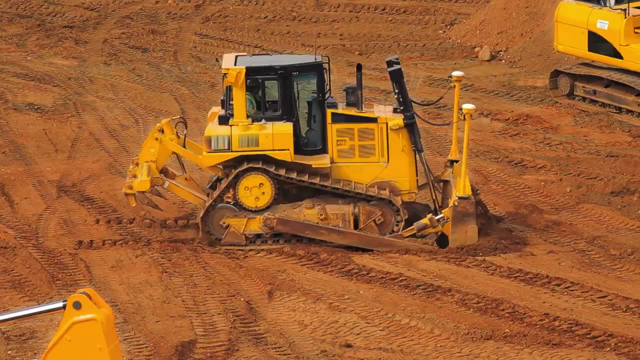 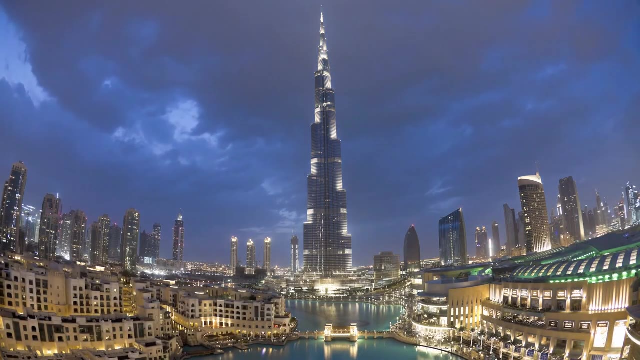 behavior. This essential process plays a critical role in ensuring the safety, cost-effectiveness and environmental sustainability of construction projects. By examining the soil and rock beneath our feet, engineers can design structures that stand the test of time and withstand the forces of nature. And that's all for today's episode. Thank you for. 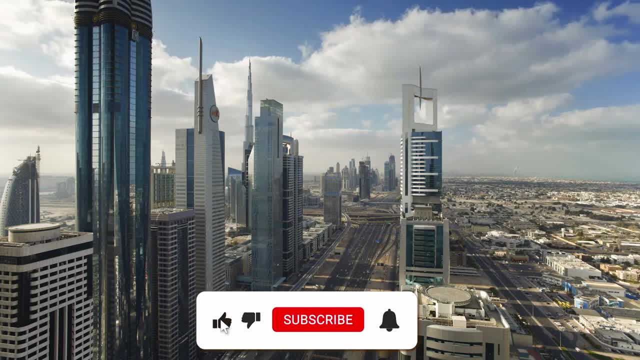 joining us. If you enjoyed this video, be sure to give it a thumbs up, and don't forget to subscribe for more upcoming videos. Till then, peace out. 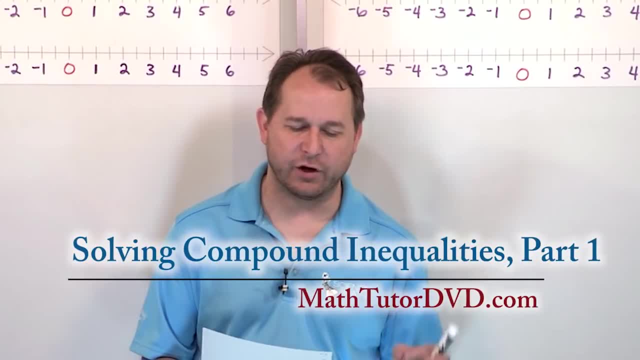 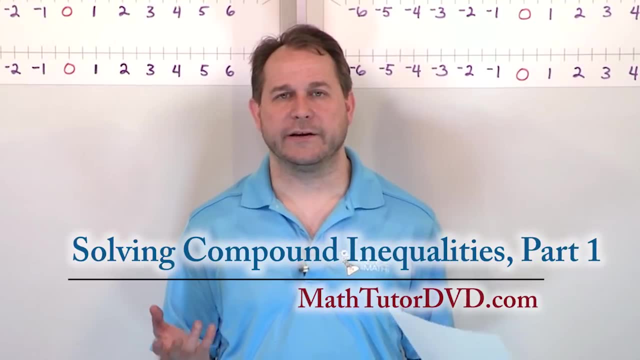 Hello, welcome back to Algebra In this lesson. the title of this lesson is called Solving Compound Inequalities. This is part one of several, So in the last section we learned how to solve inequalities generally, And it was pretty easy to be honest with you once. 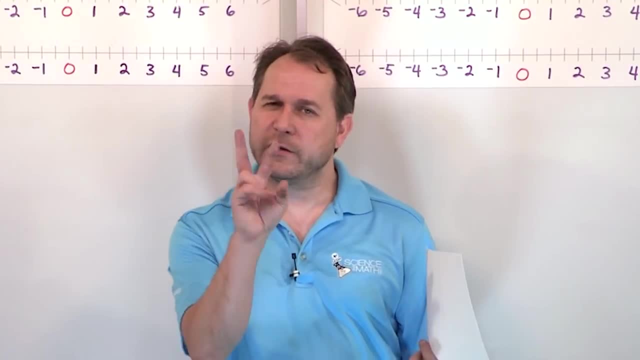 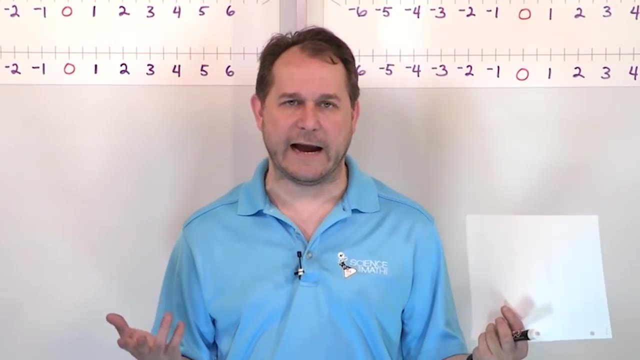 you get the hang of it because it's exactly the way that we solve equations. We had the one little rule about flipping around the arrow, but other than that it was the same. Then graphing the inequalities became pretty easy once we showed you exactly how. Now in 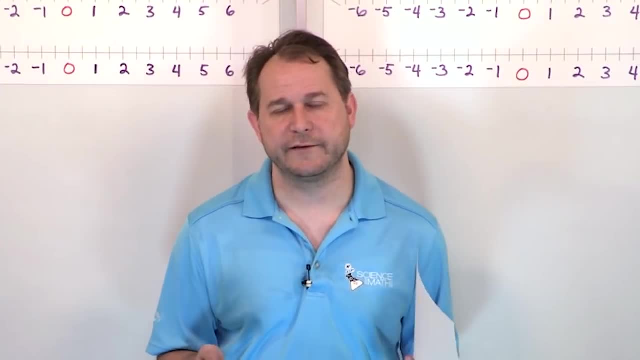 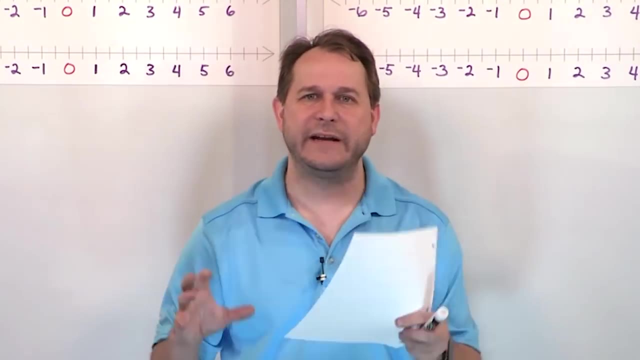 this lesson you start to get to the point where some students start to get a little lost. There's no good reason for it, though It's not difficult, But when we solve compound inequalities, we start taking the idea of inequalities and bolting on more stuff to. 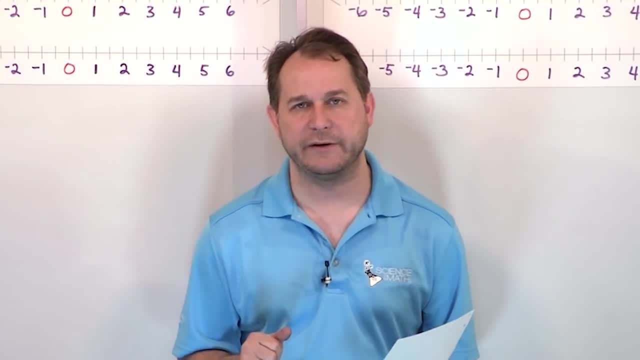 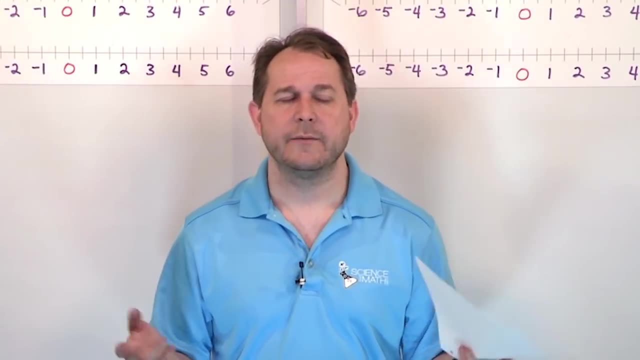 it All right. so the bottom line is there's two kinds of compound inequalities. There are inequalities that involve and the word and. They're called conjunctions, because and is a conjunction in English, The word and is what we call a conjunction. And then 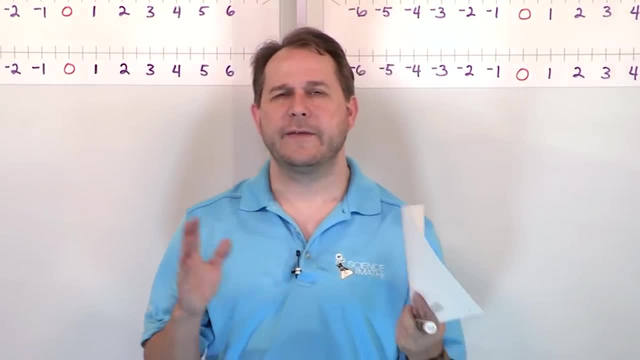 we have disjunctions which are used with the word or, So the word or is a conjunction in English And the word or is a conjunction in English. So the word or is a conjunction in English And the word or is a conjunction in English.